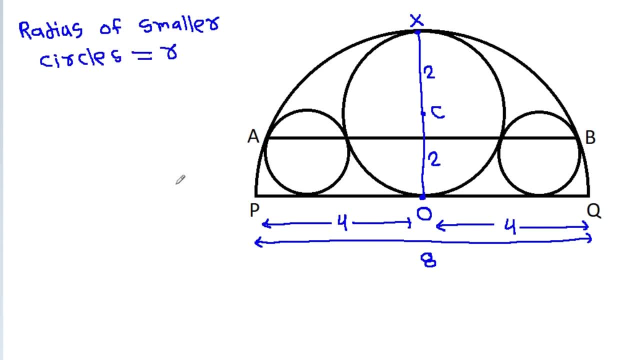 That will be 1. is equal to R, and suppose center of this circle is M and suppose this point is N, then MN, it will be R, and if two circles are touching each other and if we join center of both the circle then it will pass through common point of contact. so if we join M and C then it will pass through. 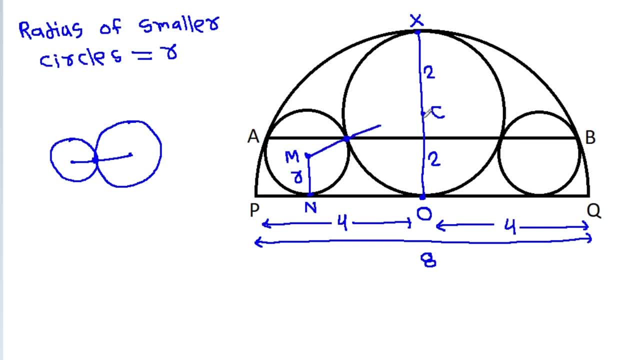 this point and now in MNOC it is M N, O C. suppose this point is Y, then MY it will be R and CY it will be 2, so MC it will be 2 plus R and MN it is R, and if we draw a perpendicular from M on CO, 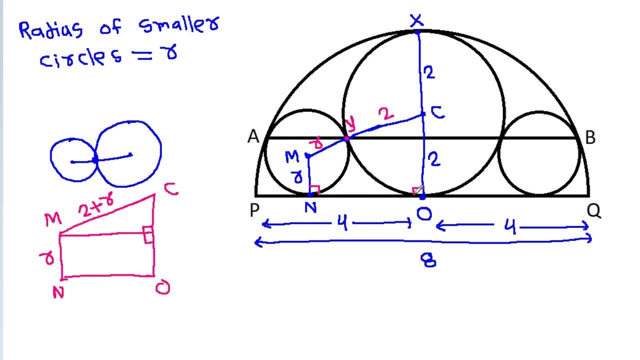 then radius and tangent, they are perpendicular to each other. so these two angles, they will be 90 degree, and suppose this point is D, so MnOd it will be rectangle, so Od it will be R, and we have Co is 2, that means Cd, it will be 2 minus R. 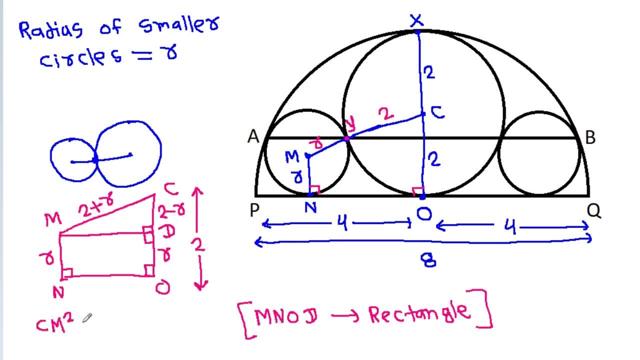 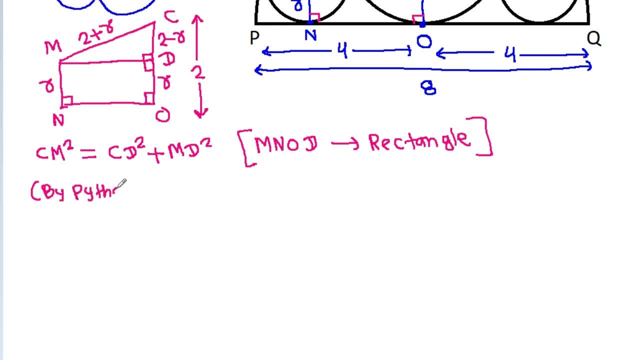 and Cm square, it will be equal to Cd square plus Md square by Pythagoras theorem. and Cm is 2 plus R square, it is equal to Cd is 2 minus R square plus Md square, and it is 4 plus R square plus 4R. 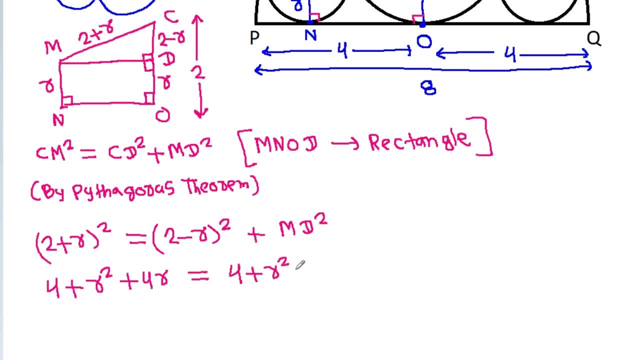 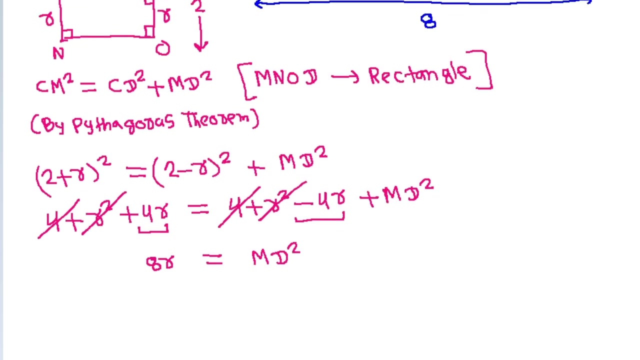 is equal to 4 plus R square minus 4R plus Md square, and 4 plus R square, it will get constant and 4R plus 4R will be 8R. that is equal to Md square, so Md it will be equal to. 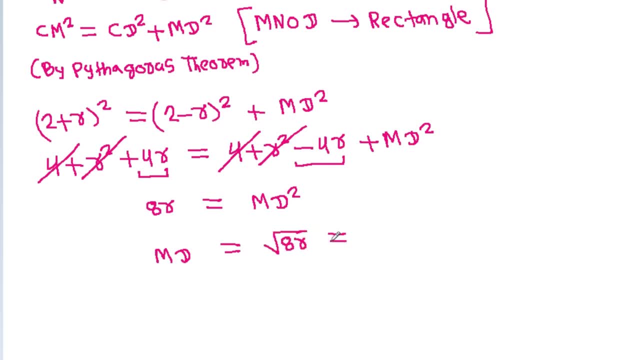 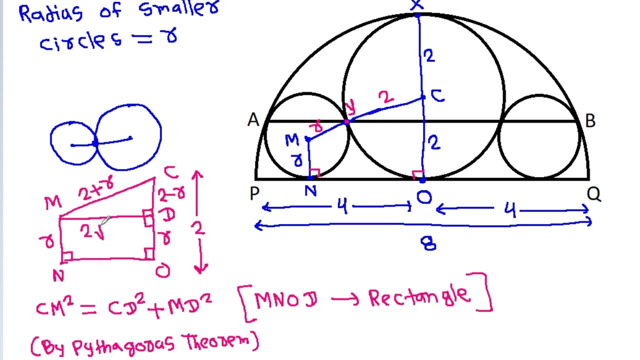 a square root of 8R, that will be equal to 2 times a square root of 2R, Md. it is 2 times a square root of 2R and Md. it will be equal to No. it will be equal to 2 times a square root of 2R. 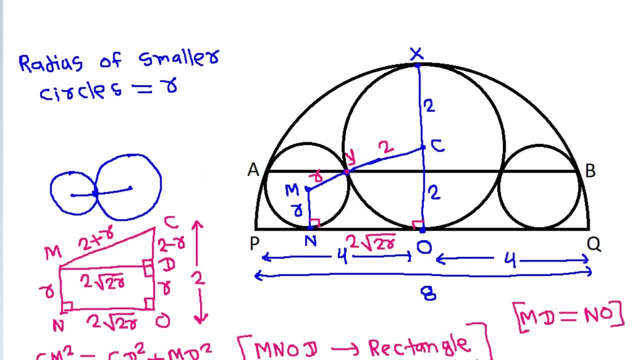 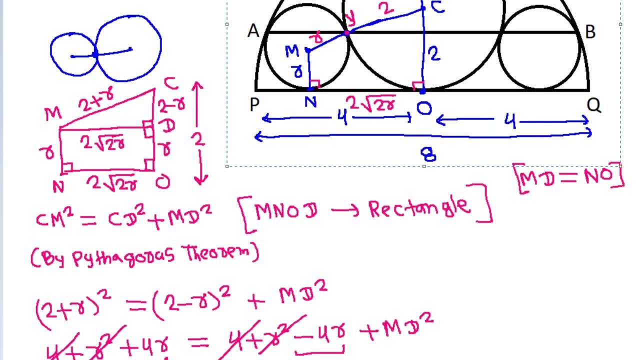 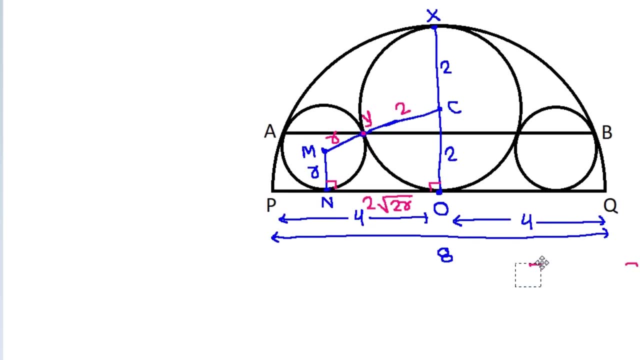 and it will be equal to 2 times a square root of 2R. Now if we join OM, then OM it will be equal to OA minus MA And OA it will be 4 minus MA will be R. So OM it is 4 minus R And inter angle MNO. 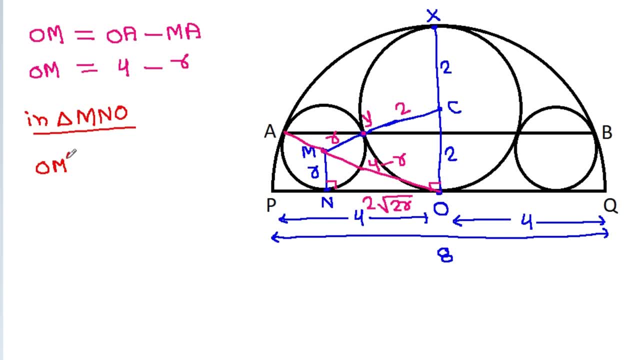 OM square it will be equal to MN square Plus ON square by Pythagoras theorem. And OM is 4 minus R square it is equal to MN is R square plus ON is 2 times S square root of 2.. So OM is 4 minus R square. 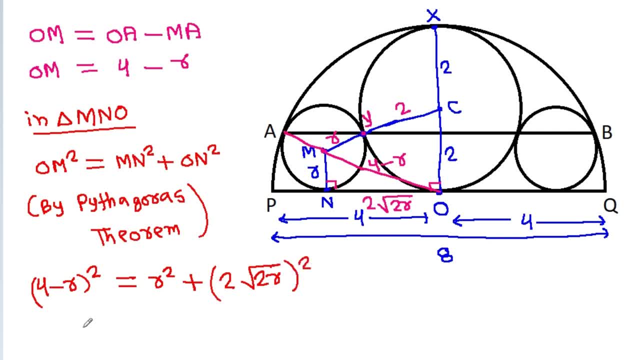 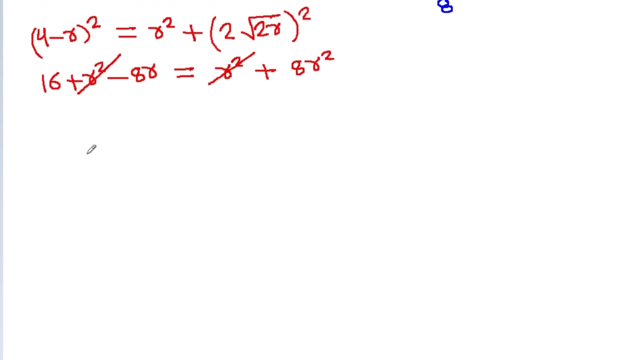 So OM is 4 minus R square And it is 16 plus R square. minus 8R is equal to R square plus 8R square And R square will get cancelled. So it is 8R square plus 8R square. 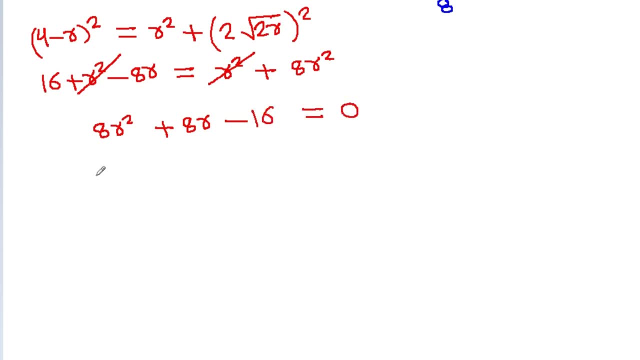 So it is 8R square plus 8R square minus 16 is equal to 0.. And it is 8 times R square plus R minus 2 is equal to 0. So R square plus R minus 2, it will be equal to 0.. 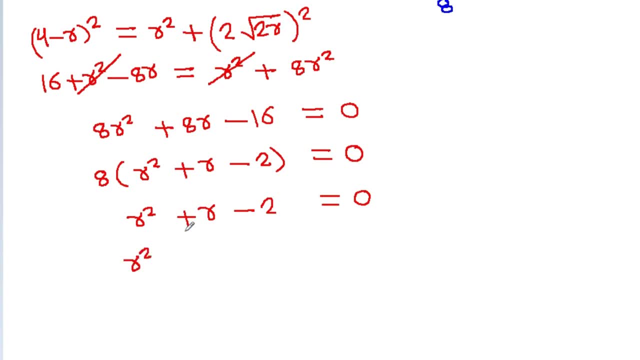 And it is R square and plus R, it is plus 2R minus R minus 2.. That is equal to 0.. And it is R times R plus 2. minus times R plus 2 is equal to 0.. And it is R minus 1 times R plus 2 is equal to 0.. 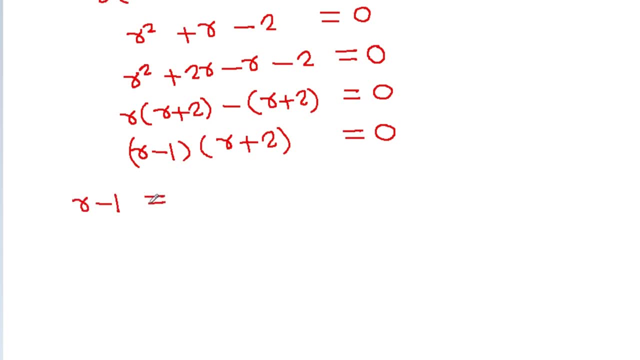 So either R minus 1, it will be equal to 0. That means R is equal to 1.. And either R plus 2, it can be equal to 0. So R will be equal to minus 2.. 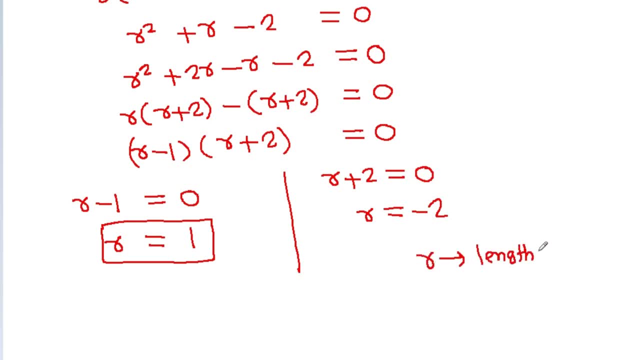 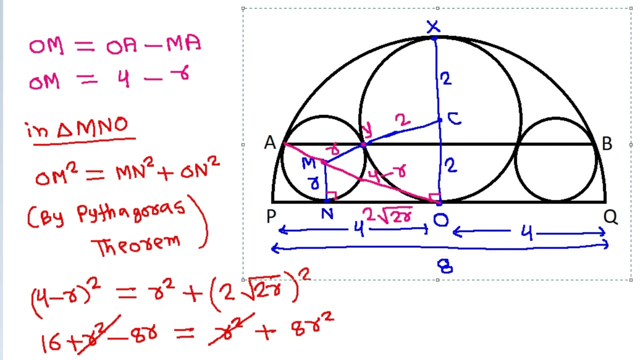 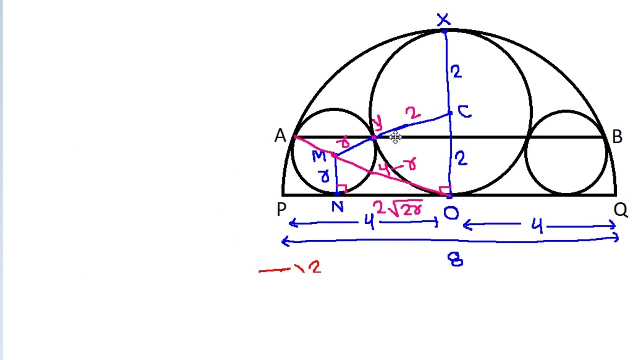 But R is length. That should be positive. So it is not possible. So we get R is equal to 1.. And now we get R is equal to 1. So we get R is equal to 1.. 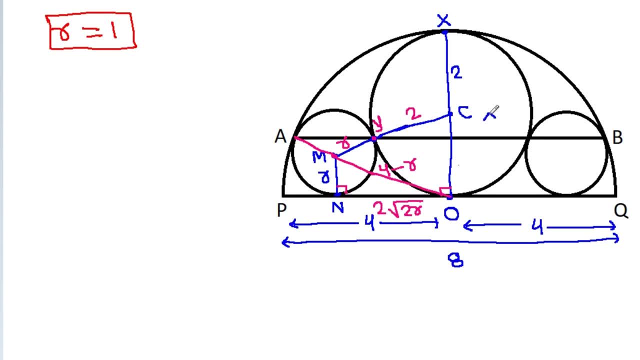 We have CO is 2.. And if we draw a perpendicular from M on CO- suppose this point is D And suppose this point is E- Then triangle CEY, it will be similar to triangle CDM. that means CE by CY, it will be equal to CD by CM. 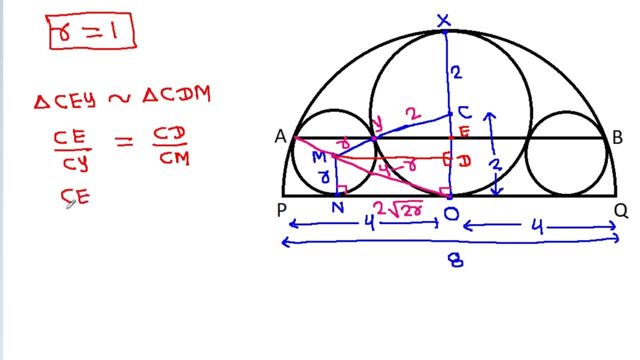 and CE. by CY is 2, it is equal to CD. by CM is 2 plus R and CE by CD, it will be equal to 2 by 2 plus R is 1, that is equal to 2 by 3.. And OD it will be equal to NM, that is R, that will be 1. so OD is 1 and CD it will be equal to CO minus OD. 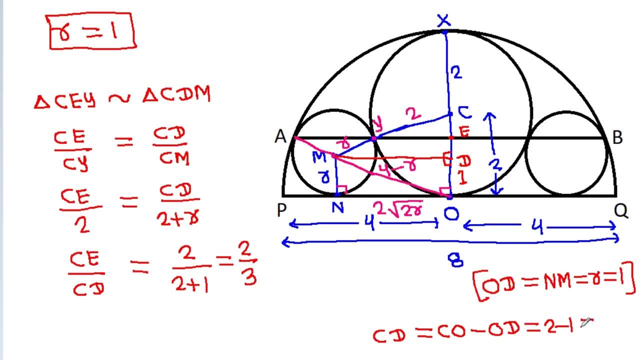 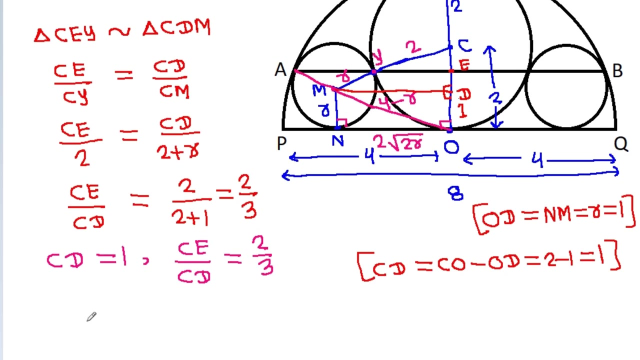 that is 2 minus 1 and it is 1.. So we have: CD is equal to 1 and CE by CD is equal to 2 by 3.. So CE by CD is 1. that is 2 by 3. so CE it will be equal to 2 by 3.. 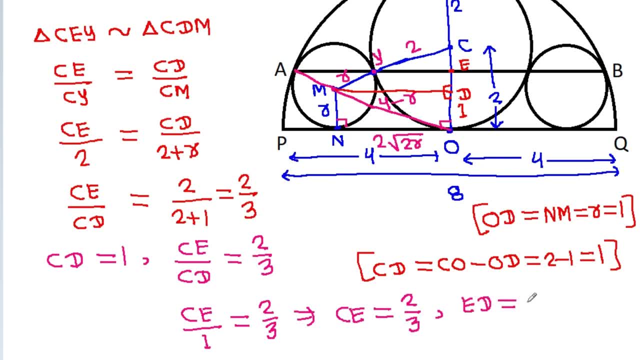 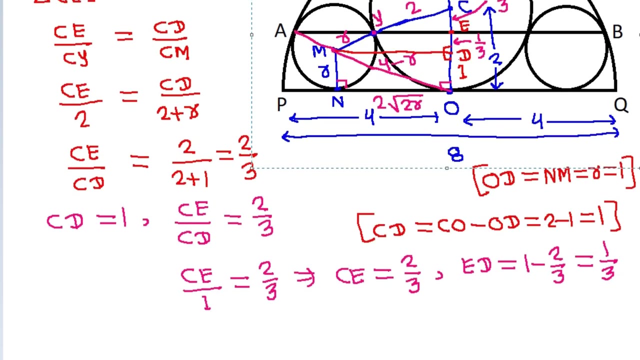 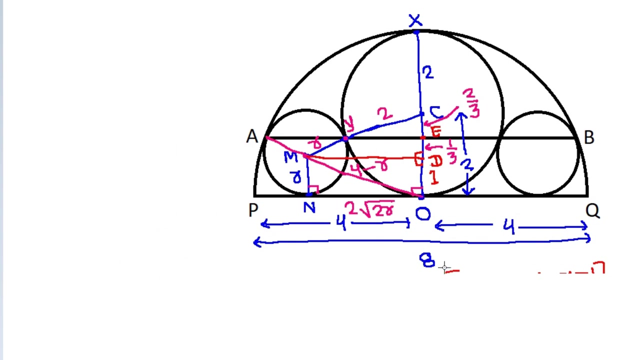 And ED it will be equal to 1 minus 2 by 3. that will be 1 by 3. so ED it is 1 by 3. And CE it is 2 by 3.. And Sub Now: if we join OB, then OB it will be equal to 4. 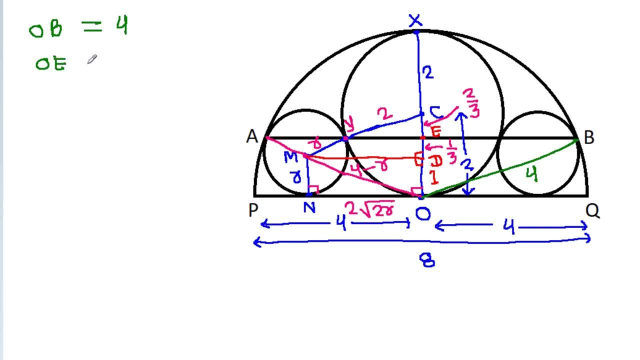 And we have: OE is equal to OD plus DE, That is equal to 1 plus 1 by 3.. That is equal to 1 plus 1 by 3.. and NM is equal to 0.. and it is 4 by 3.. So inter angle OEB, it is OEB. this angle will be 90 degree by symmetry. 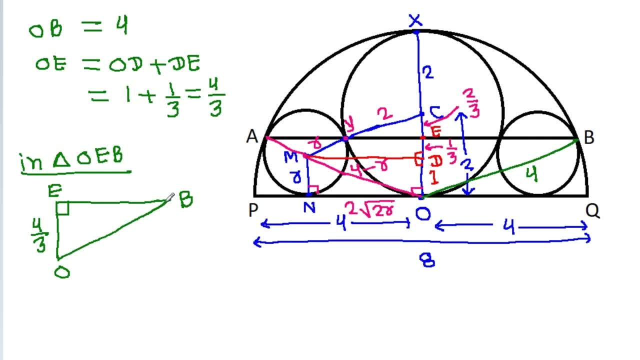 and OE is 4 by 3, OB is 4.. So EB square: it will be equal to OB square minus OE square and it is 4 square minus 4 by 3 square that is equal to 16 minus 16 by 9 and it is 8 times. 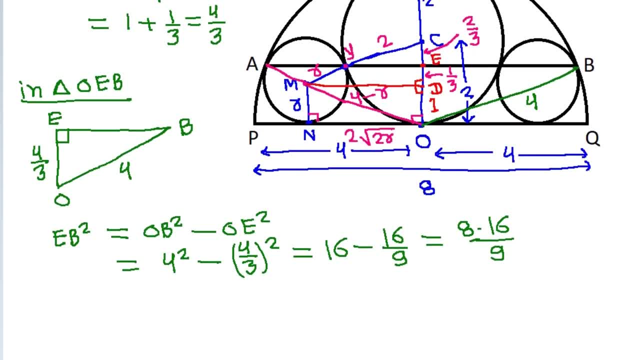 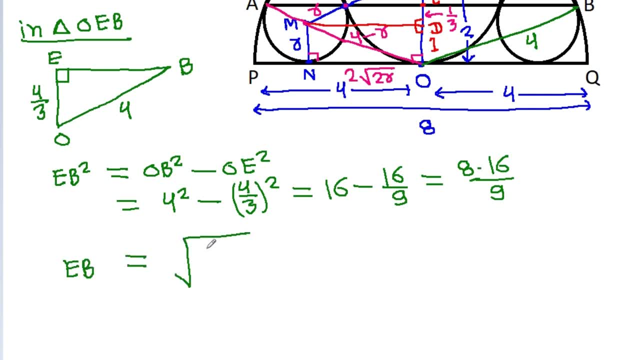 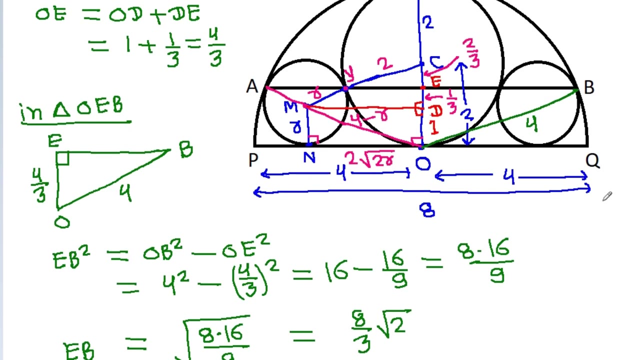 16 by 9.. So EB it will be equal to S square root of 8 times 16 by 9, that will be equal to 8 by 3 times S square root of 2.. EB: it is 8 by 3 times S square root of 2.. 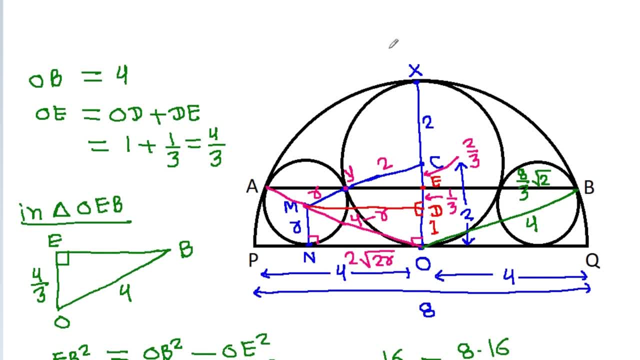 Thank you And AB. it will be equal to 2 times EB by symmetry. So it will be equal to 2 times 8 by 3 times S square root of 2.. That will be equal to 16 by 3 times S square root of 2..